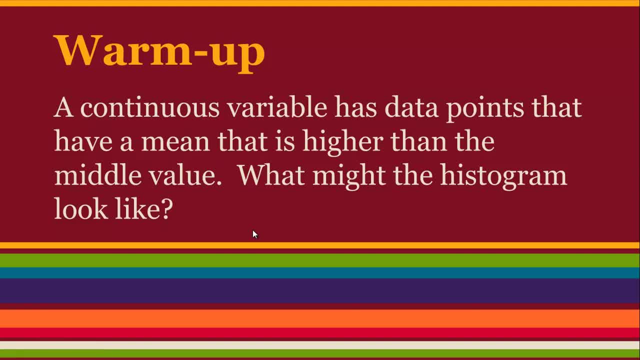 The mean is pulled to the right. We're going to get to that in the stats unit, but I just really wanted to see if you could remember what drawing a histogram might look like. Okay, so the Learning Target. we're going to cover this in this video. 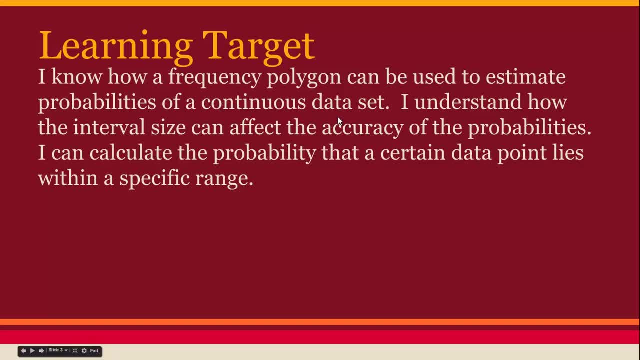 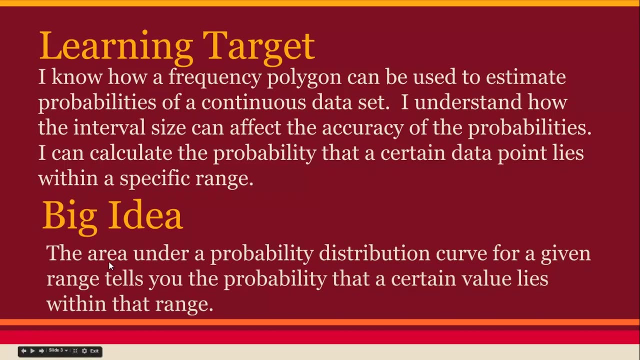 I know how a frequency polygon can be used to estimate probabilities on a continuous data set. Okay, So we can understand how the interval size can affect the accuracy and I can calculate the probability that a certain data point lies within a specific range. The big idea is the area, and this is what we're really going to get to. 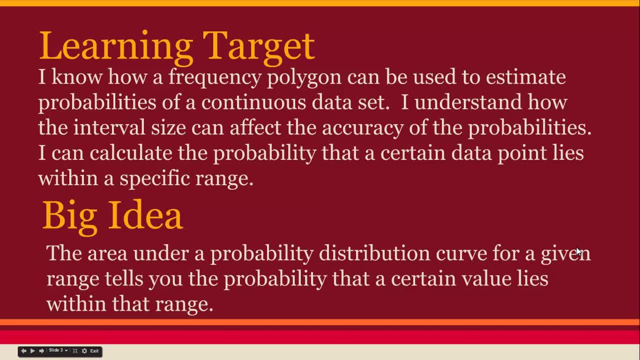 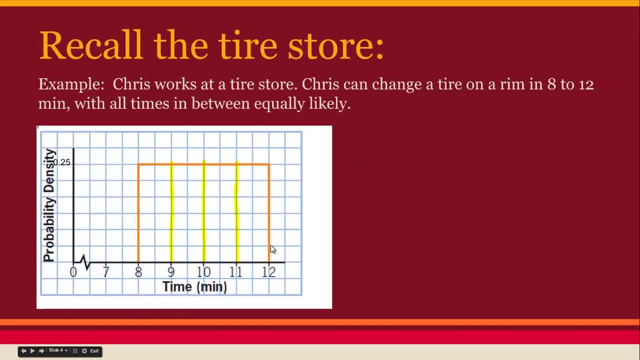 the area under a probability distribution curve for a given range tells us the probability that a certain value lies within that range. So today is going to be all about calculating area. So we saw this before. Like Chris has the tire store. What is the relationship between the area of the rectangles and the probability of each? 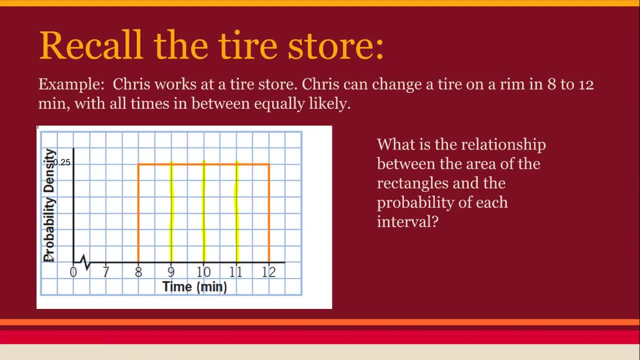 This word probability density. this is actually a key. This is a probability density histogram. This is four bars. This actually the area is calculated, or the probabilities are calculated by calculating the area. So I can go from like 9 to 9.5 and just really calculate that area as length times width or base times height. 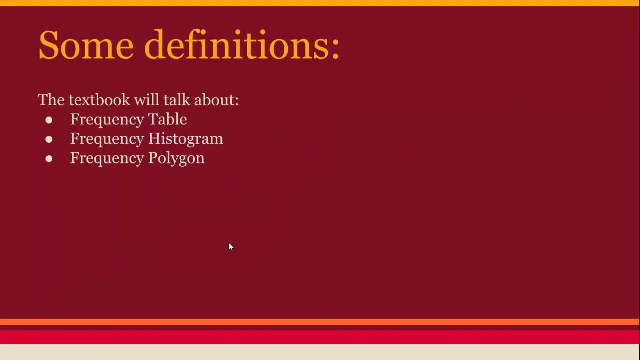 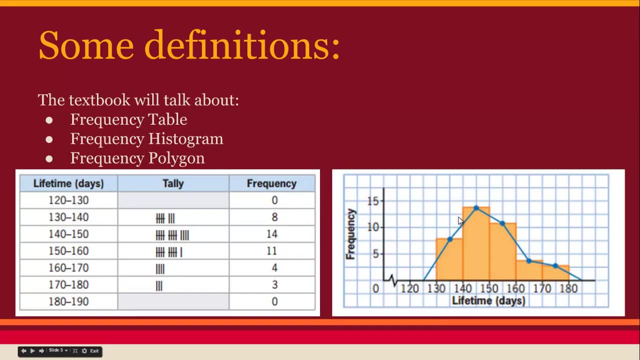 So the area just tells us. the probability Textbook talks about frequency table, so how many times something comes up? A frequency histogram, which is the orange here, and a frequency polygon, which is really just a sided figure. It connects the midpoints of the data. 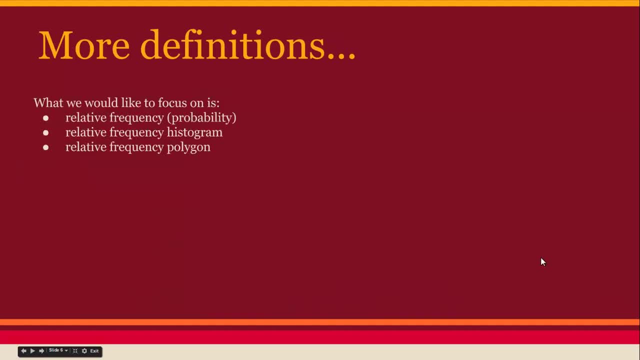 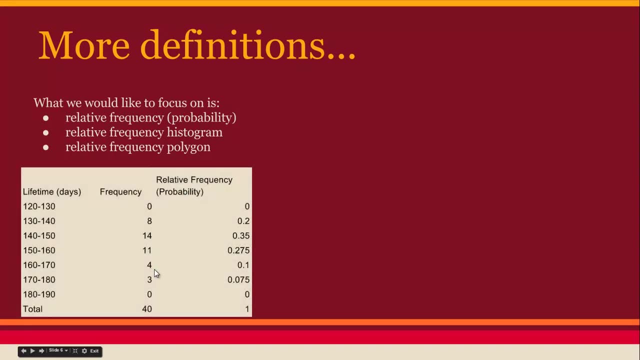 So that's what a frequency polygon looks like. What we want to focus on is a relative frequency, so we really care about probability. A relative frequency histogram, A relative frequency polygon. So here we actually have like an interval size of 10.. 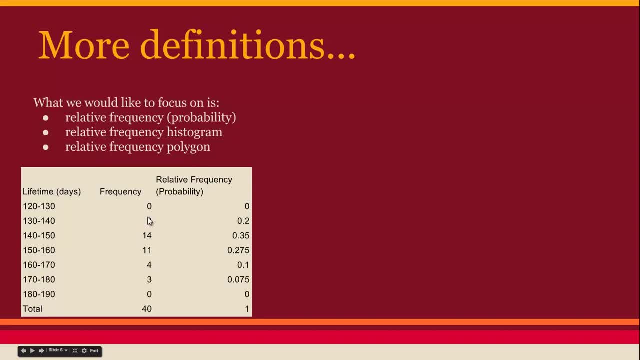 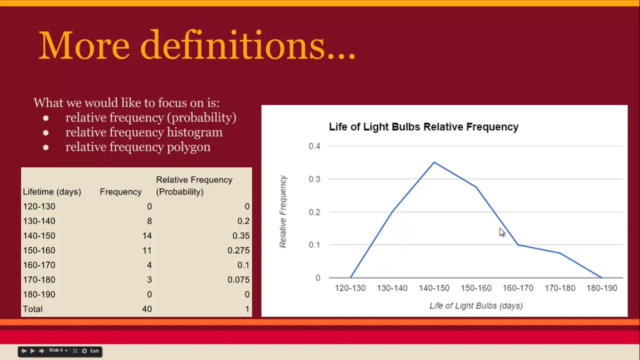 Probabilities are just calculated by dividing the frequency by the total, which is 40.. And the probabilities will add up to 1.. The area under this curve. this is a relative frequency graph. The area under this curve does not add up to 1.. 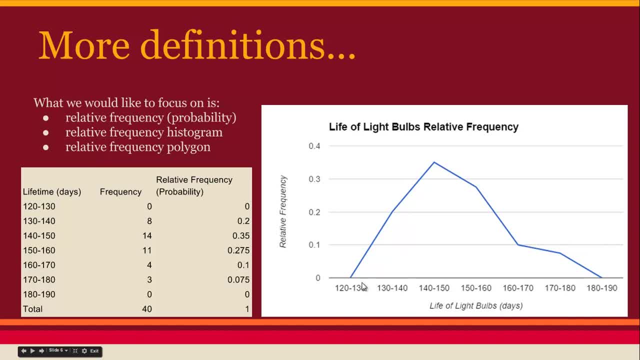 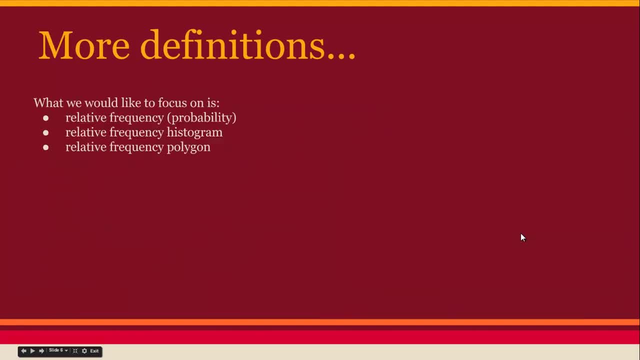 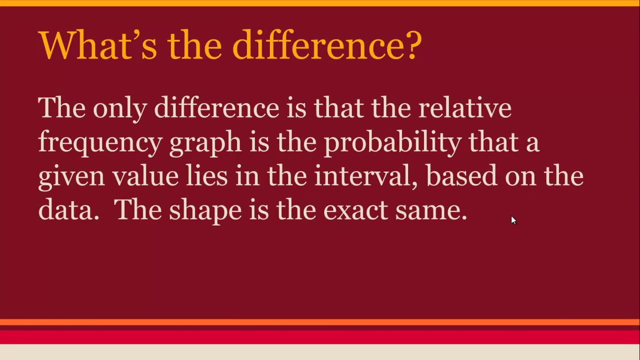 The area under this curve adds up to 10.. Because the? Because the interval size is 10.. But notice that they are the exact same shape. This here polygon and this polygon are the exact same shape. So what's the difference? The only difference is the probability that a given value lies in. the interval is based on the data. 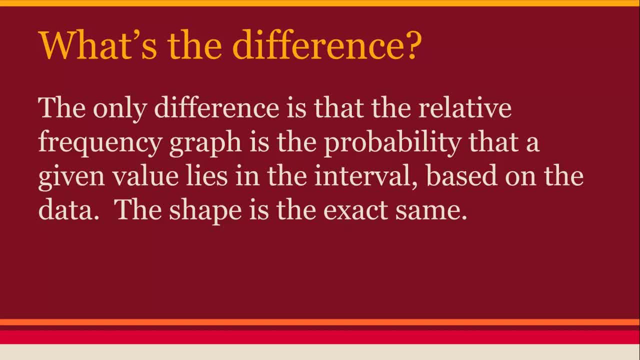 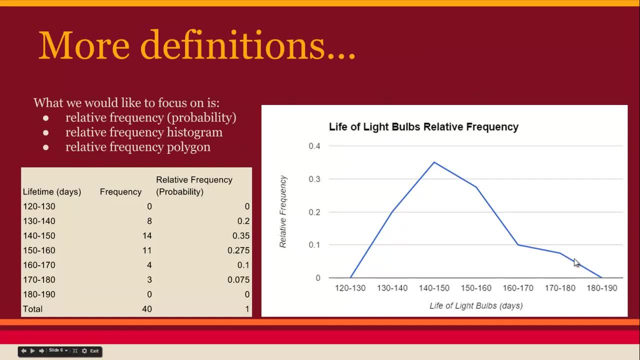 So, like, instead of frequency, we've got probability and the shape is the exact same. But we are waiting for that idea of calculating the area under the curve, which can't be done here. But you don't need to Like, you've already got the probabilities. 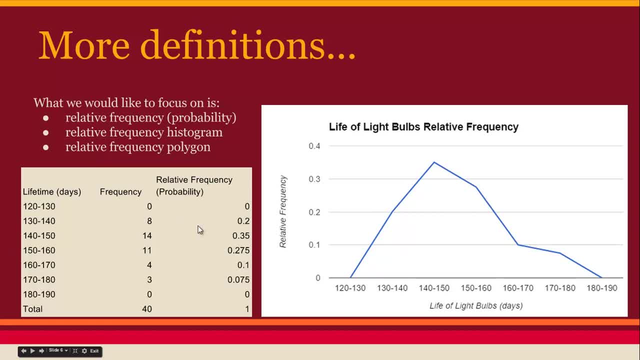 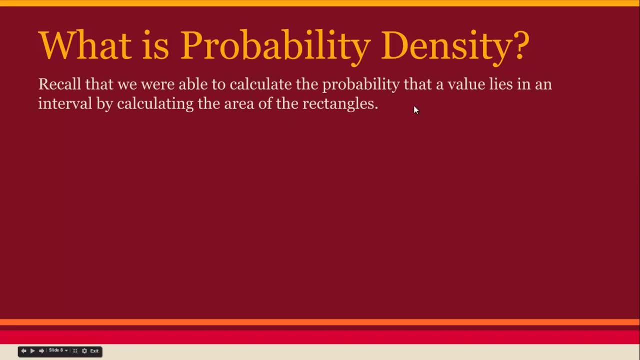 We already know the probability that you lie in certain intervals. Okay, What is the probability density? Recall that we were able to calculate the probability that a value lies in the interval by calculating the area of the rectangle. So we did this with the tire shop. 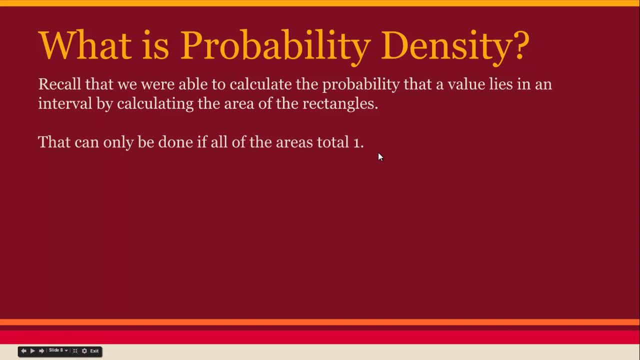 It can only be done if the areas add up to 1.. So that's not always the case. So probability density areas do add up to 1.. When the interval size is 10, that can't happen. Okay, So it's just if the probabilities add up to 100%, but the interval size is 10, that doesn't work. 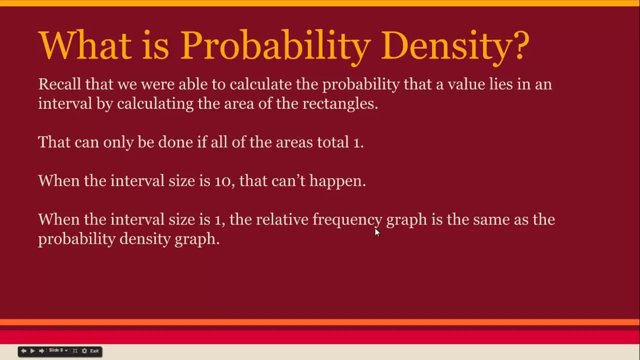 When the interval size is 1, it does happen. Relative frequency graph is the same as probability density. If you don't have relative frequencies- or sorry, if you have the relative frequencies- you don't need a probability density, though. That's the key. 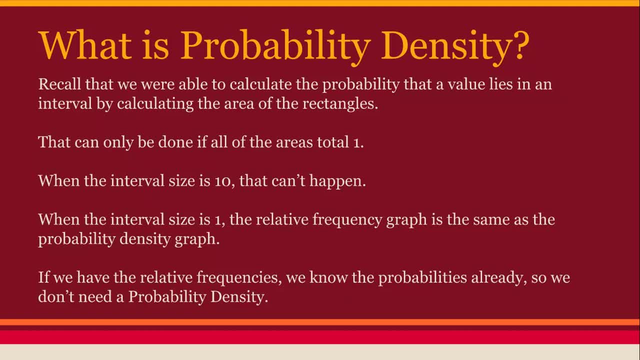 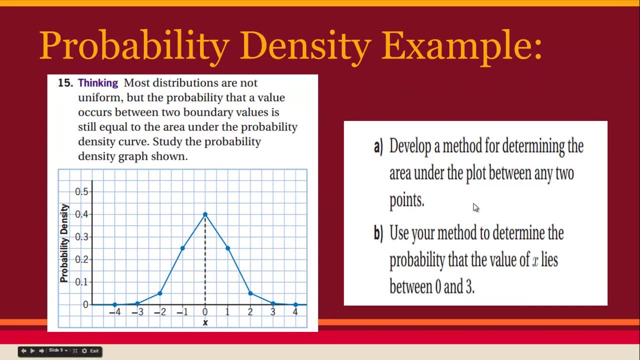 So you don't need to go area under the curve, unless you want to get more accurate than an interval size of 10.. So here's a question for you. I'd like you to take some time to do this. You're just actually calculating the probability. 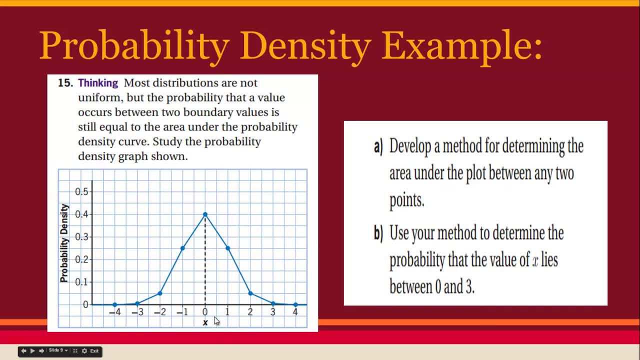 This is the probability density, So we're going to take the area under the curve between 0 and 3.. So I'm going to take some time to do that. The method that a lot of people use is like just taking rectangles. 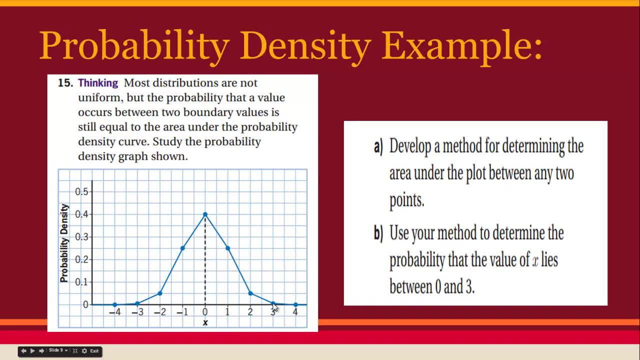 Some people like calculate the area of the triangle, You notice that that 3 is really just off the axis, So we have to estimate where that is. Okay, Okay, Okay, Okay, Okay. What the method we're going to use eventually is is to actually calculate areas of rectangles. 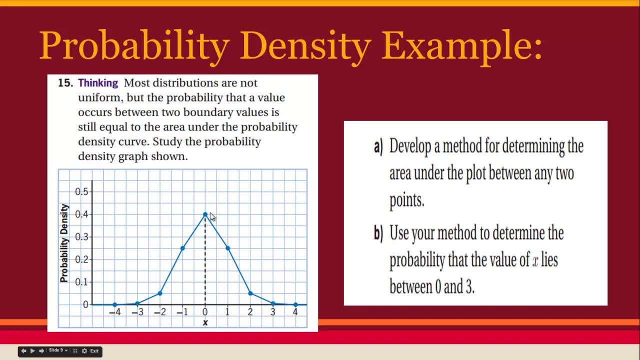 And we're going to see that in the next lesson which I'm going to show you right now. Okay, So if we actually just calculate the area of rectangles, the area of those rectangles, they are going to kind of overlap, Like there's going to be a little bit of a rectangle that's going to come out, because this is a straight line coming down. 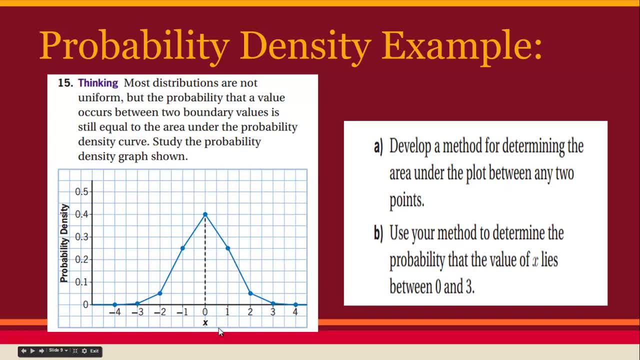 But where we overcount area, we're actually going to get a little bit of a rectangle that's going to come out, And then we're actually going to undercount area as well. So that's going to be the method we're going to use to find the area. 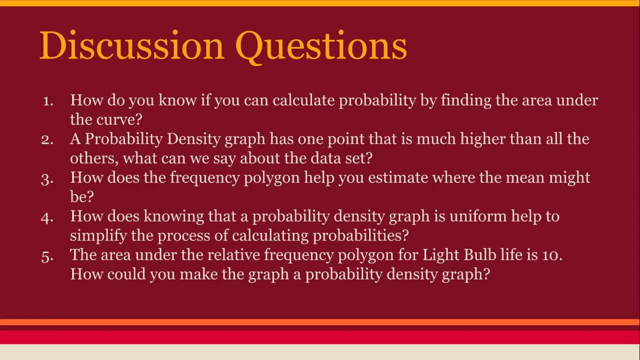 Some discussion questions. These are just really to think about. If the area is 10,, what we could do is just divide all the probabilities by 10.. And that's what we're actually going to see in the next one. Hows the frequency polygon help you to estimate the mean might be? 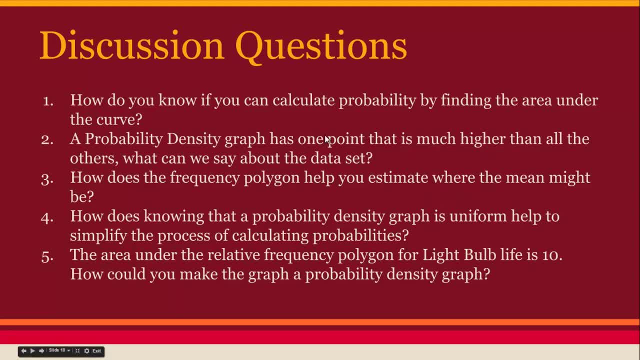 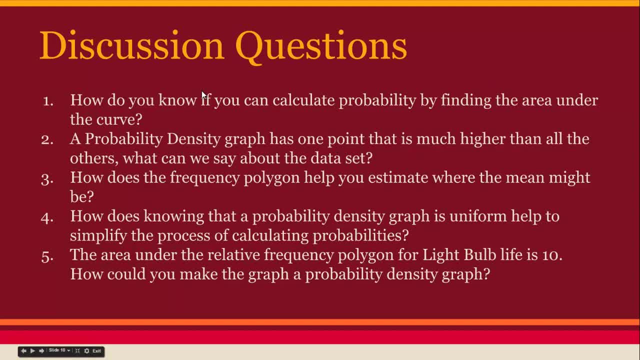 calculate? reflection question: if the, if they add up to one, if the interval size is one, how does a frequency polygon help you to estimate where the mean might be? probability density graph. so I just really want you to think about the data I was knowing. the probability density graph is uniform. help to simplify the. 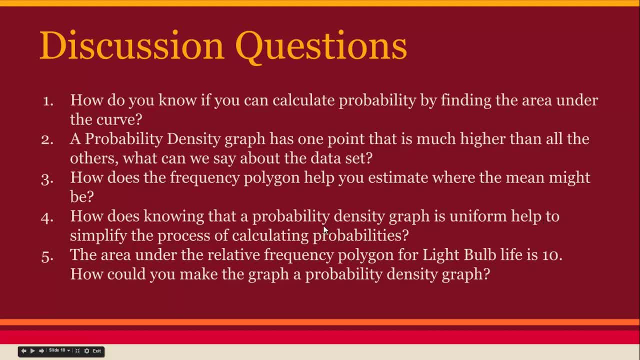 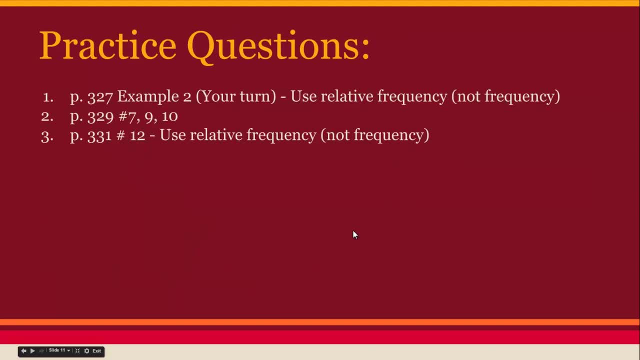 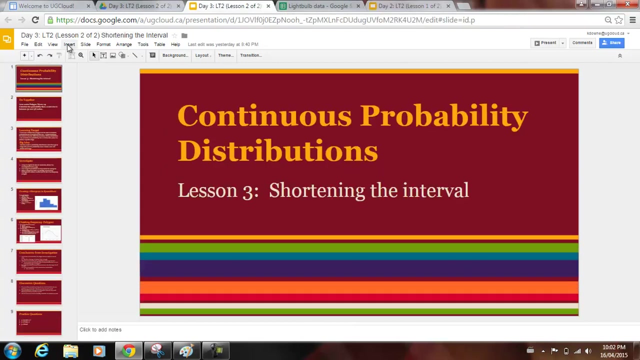 process. a uniform distribution is the easiest one to calculate. it's just a rectangle, and so that was Chris's tire store. it's very easy to calculate. so there's some examples here and I just want you to practice using relative frequency here, not, not, not frequency. okay, moving into lesson two, shortening. 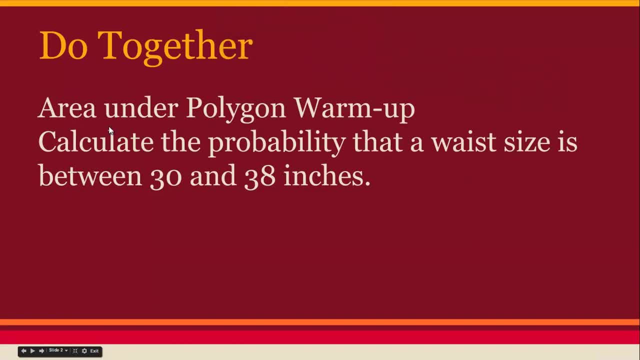 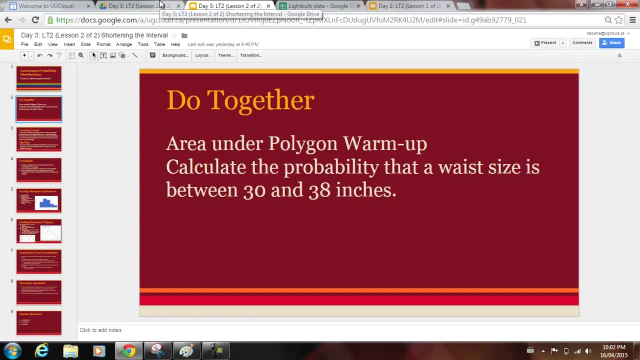 the interval. try this question: the area under polygon warm-ups, we're gonna calculate probably the way. size is between 30 and 38. to share with you how to do this, if you can't, if you don't have the handout, if you don't have this page, if you don't. 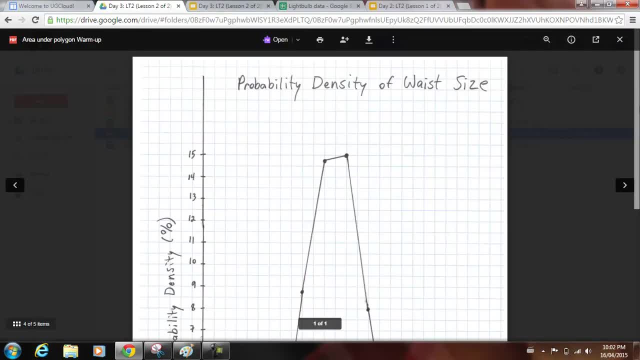 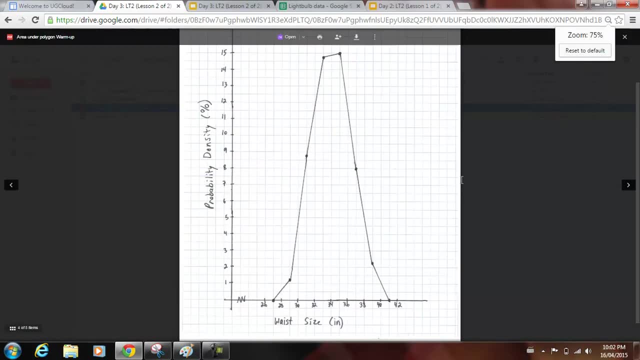 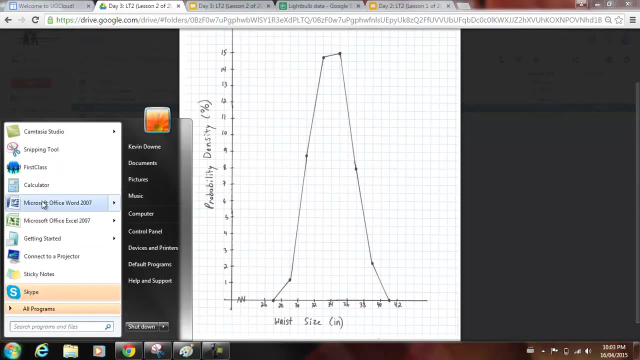 print off this page. but this is what we're looking at here, probably density of waist size, and so we've got this, this picture of the curve, and this is probably density. so we'll tell you the area under the curve there's something that Windows has called the snipping tool. when you open it, it will. I've got this. 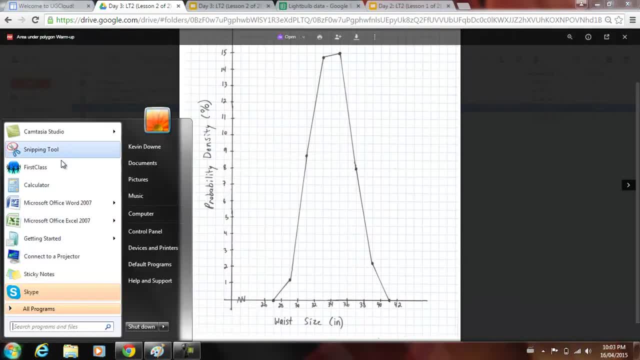 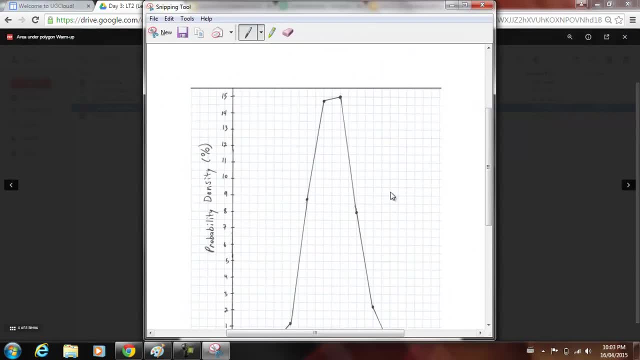 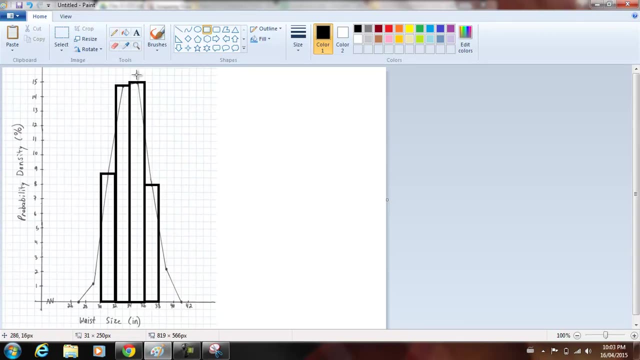 open already. I'll just show you. it's a very handy tool for copying and pasting. so if we can, we can just highlight anything. we can paste it into a report. so if we say edit copy here, I'm actually just gonna paste it into paint, and so I. 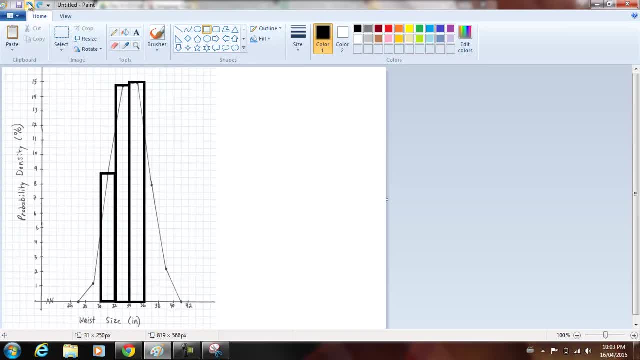 could actually draw some rectangles on there. why show you the rectangles out we drew? so question asks us to find the area under the curve between 30, which is down there two thirty eight, and so the method to do that is just draw these rectangles. and so if we see that area between 30 and 32, 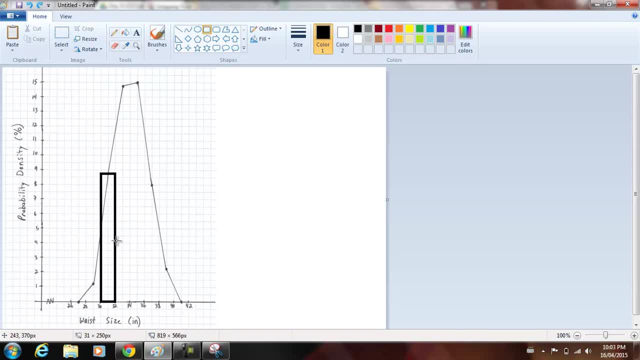 this is a little less time- is a good estimate for the area. the probability we just do length, which is two times the height, which is just about me, point eight and then so that number, and it's eight point eight percent times two, so you got about seven like seventeen point six percent right there and that's. 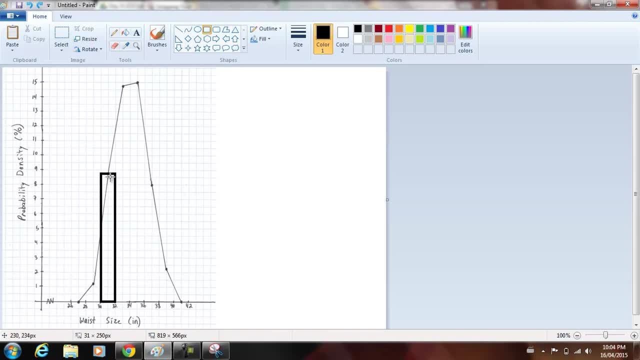 the probability that you're between thirty and thirty two. the problem is, you are overestimating the probability. you see this little part here, but don't forget like this is not an exact science anyway. so it's so to like say: well, better method would be to like: cut it here and then, when they're the triangle, 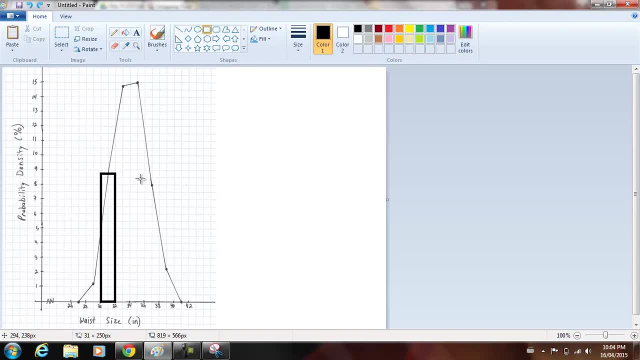 or something, or find the area of this triangle, subtract it off. but it's not exact science. anyway, we need to do an estimate anyway. notice the next rectangle. we actually don't calculate this triangle and then we do calculate another extra triangle. so it's a little so it's so. it's still not accurate. 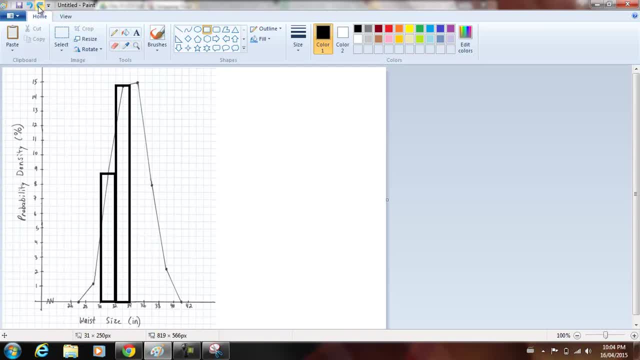 because we've got two extra triangles and we're not counting another one. a little bit more accurate, as you do more, like you know, you're counting an extra triangle, so you're counting three and then not one, and then the next one to get the probability between 30 and 38. we can add up the 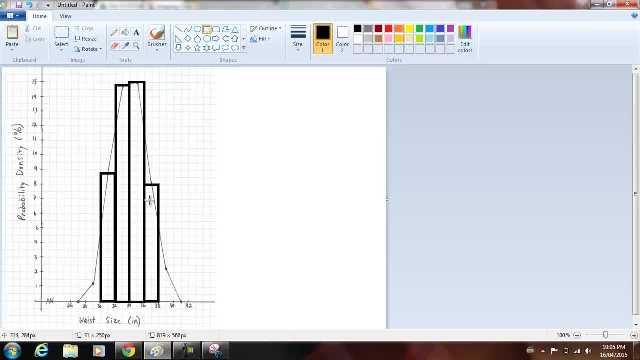 areas of all these rectangles and again there is some overlap, but then there's triangles that we're not counting as well. it's not perfect, but it is a lot easier than having to worry about areas of triangles. we're just really looking at the area of these four rectangles and that's going to give us the probability. 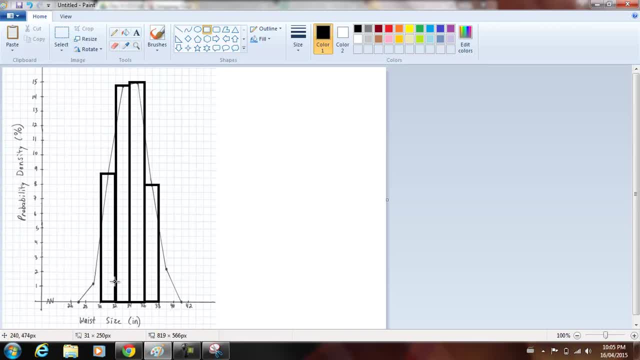 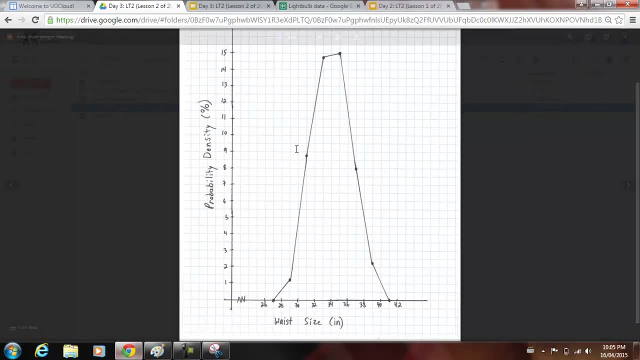 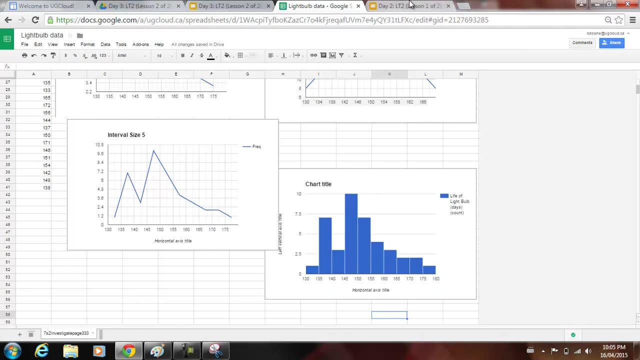 we're between 30 and 38, and so you can go ahead and do that. it's just two, and then you'd estimate the different sizes. okay, you can do that yourself, or you can do this that from this video. now I want to look at the. we'll just keep moving on. 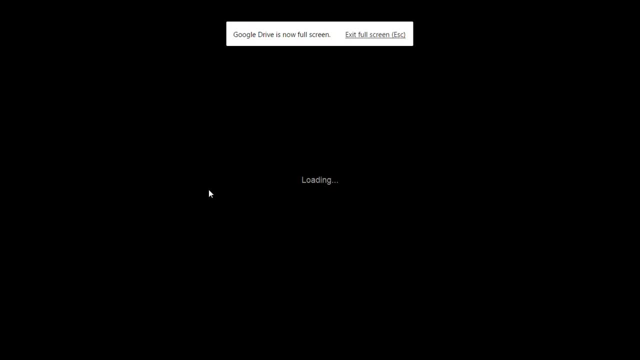 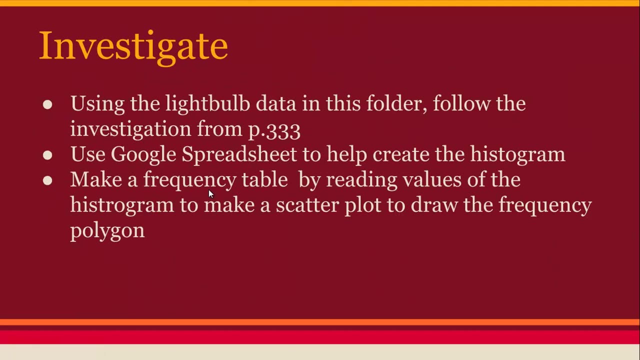 in the presentation, but this is the idea here is is just to understand this method. go back to the learning target. it's the exact same thing. we just talked about the this, the next part. I want to lead you through an investigation. it's probably a little bit more complicated than what we just talked about, but it's. probably a little bit more complicated than what we just talked about. but it's probably a little bit more complicated than what we just talked about, but it's from page 333. but really what they're asking to do from page 333, but really what they're asking to do, 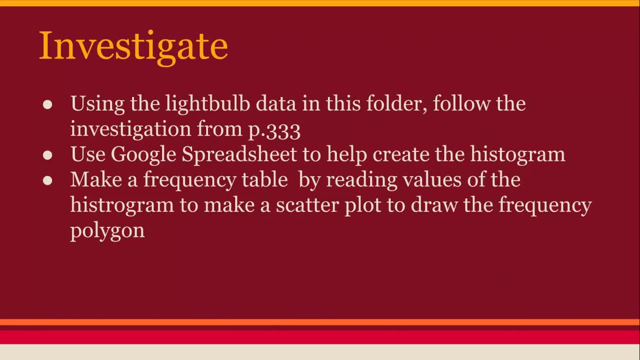 from page 333. but really, what they're asking to do is create a histogram of data. is create a histogram of data. is create a histogram of data and they give you that the interval size and they give you that the interval size and they give you that the interval size like 10, so they give you this one, that. 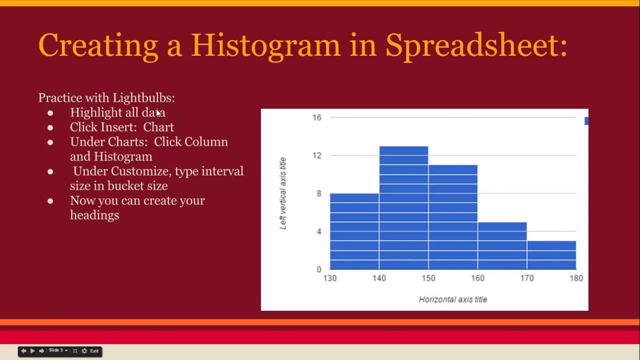 like 10, so they give you this one. that like 10, so they give you this one that I've drawn in Google Docs. I left the I've drawn in Google Docs. I left the I've drawn in Google Docs. I left the data there in the Excel sheet that's in. 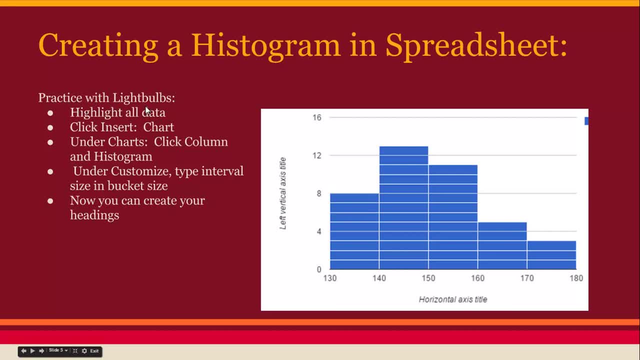 data there in the Excel sheet, that's in data there in the Excel sheet, that's in this folder and here's some directions. this folder and here's some directions actually do this, but I'm just gonna walk through it anyway. so they give you the histogram with interval length of 10, and then we'd actually draw the frequency. 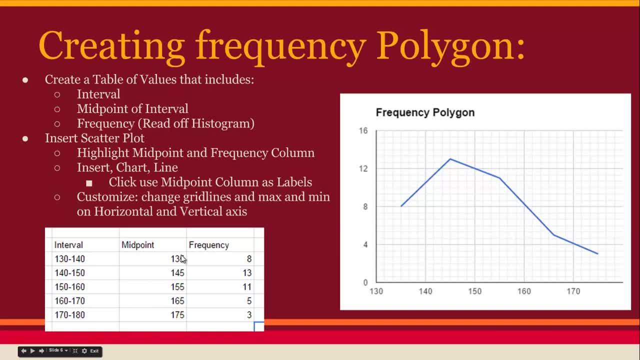 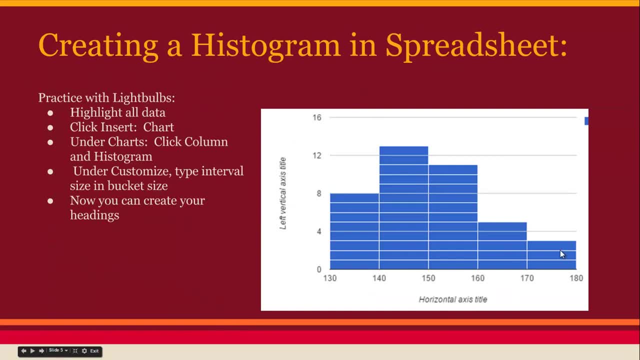 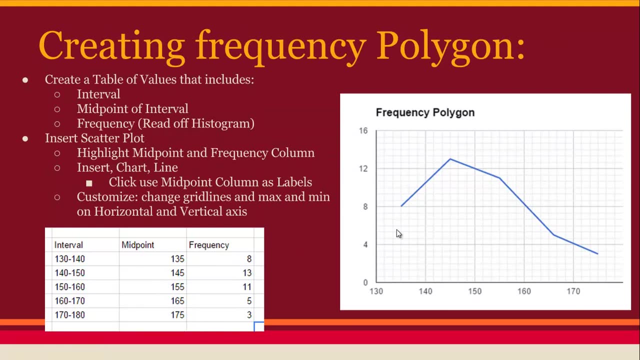 polygon we need to like, we need to set up the points, like the midpoints here, and then we had to use the frequency from the from the diagram that I just that from our histogram, so we don't actually have to count the number that are between each interval, like Google spreadsheet does it for us. and here's: 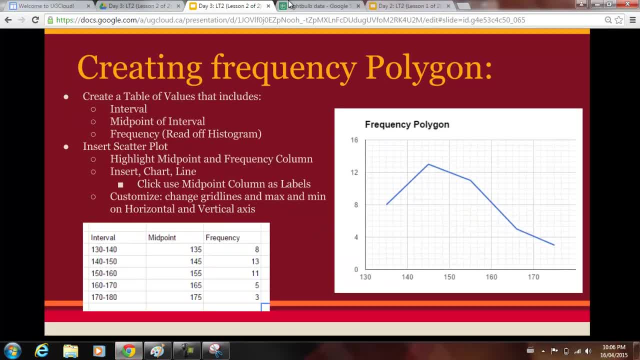 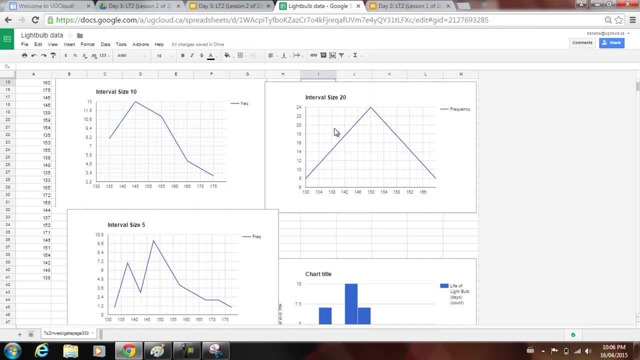 some directions for how to count, how to create it, so I'm going to show you what those, what the graphs look like, and so the point was to in in the textbook. they asked you to do it for an interval size of length: 20 in an interval size of 5. 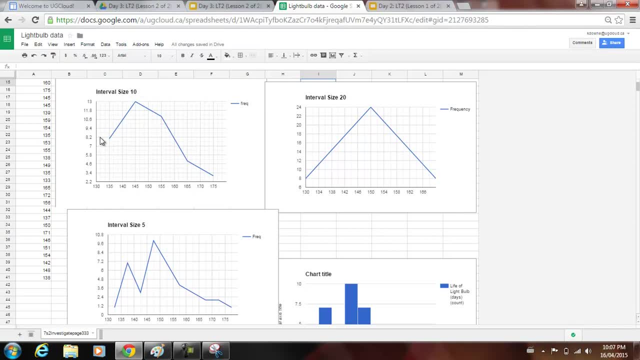 and so what happens is like, with 10, we have a certain number of rectangles we we really only have for each midpoint. so one, two, three, four, five rectangles, okay, so we're going to go ahead and do that, and we're going to go ahead, and, and we're going to go ahead and do that, and we're going to go ahead and do that. 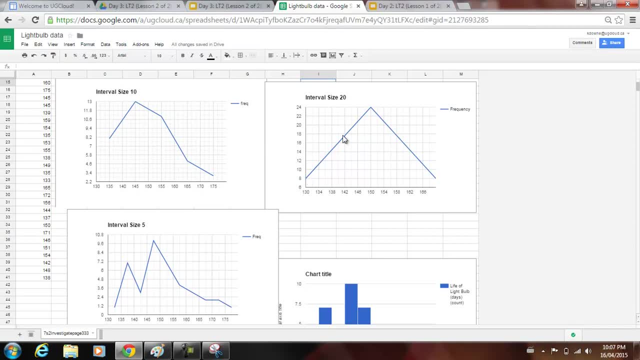 for interval size 20. we only have one, two, three rectangles interval size of five. we actually have one, two, three, four, five, six, seven, eight, nine. there should be one in here as well. so there's actually going to be ten rectangles on an interval size five, and so the question that they want to know is which. 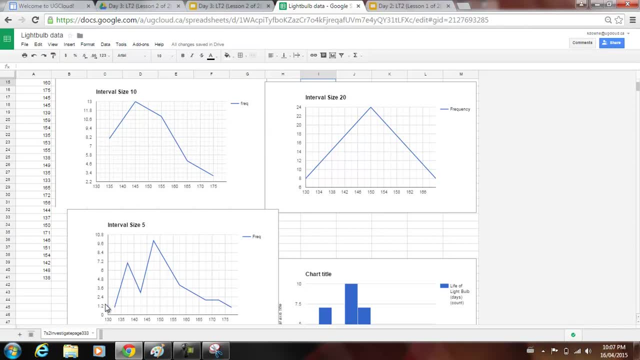 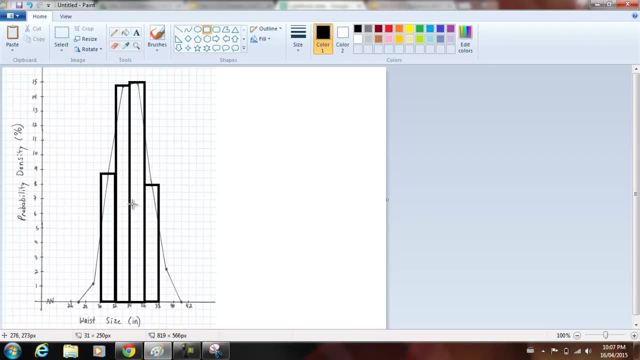 one would be more accurate and because when we do do more rectangles, you can go back to the to this guy as well. if we want to get more accurate, to do the area into the curve, we can just break this up into more rectangles. if we break this up into more rectangles, it gets more accurate. we. 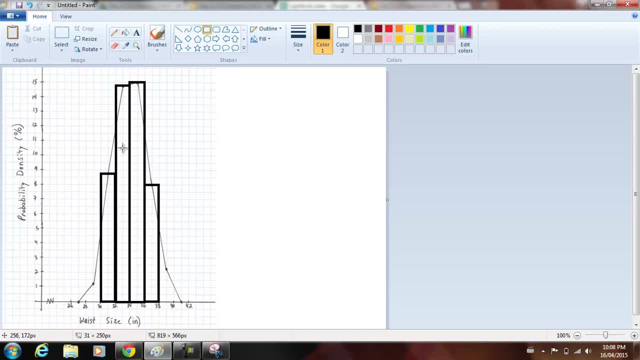 just like the rectangles are more narrow and we don't have as much of, we don't have as much like extra space that we're calculating, and so we do get lot a lot better. the problem with that is you can't always just narrow it down. so if we have a waist size inch of two inches, as 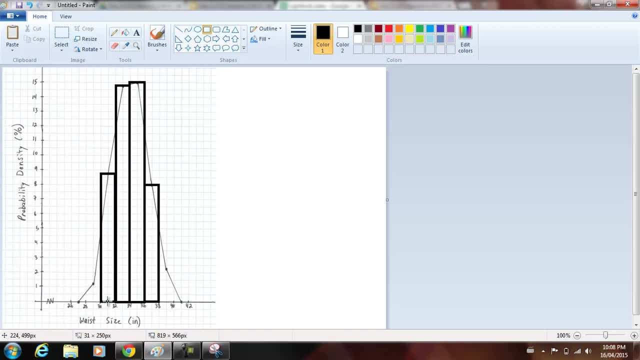 the interval. a waist size of one inch would be better. a waist size of a half an inch would even be better. quarter of an inch would be better. we just have to make sure that, number one, we're collecting accurate data. so we measure people's waist to the nearest less than a quarter of an inch. and number two, we 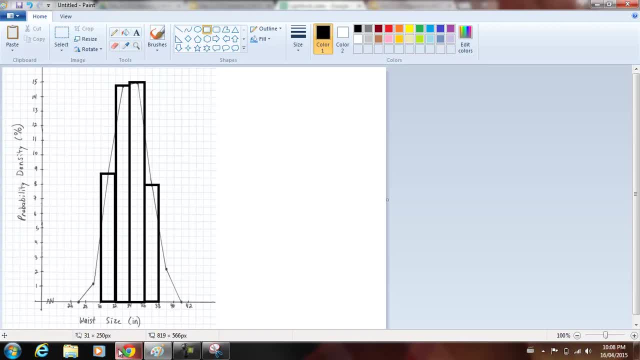 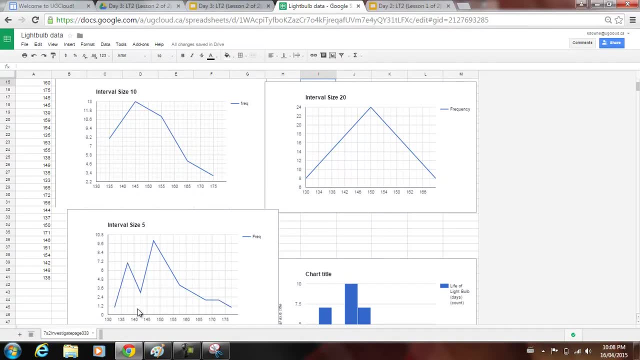 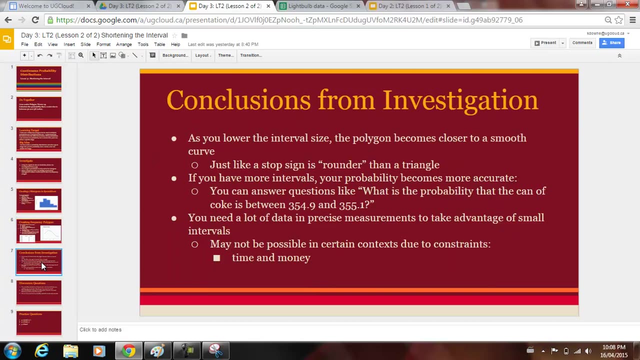 have a lot of data, because if we make a whole bunch of intervals- we saw that here- we have to make sure people are lying in those intervals as well, but it does get to be more accurate with the rectangles. okay, just a little bit of conclusion from that. so I just kind of want to wrap up, but a little bit, and remember we're 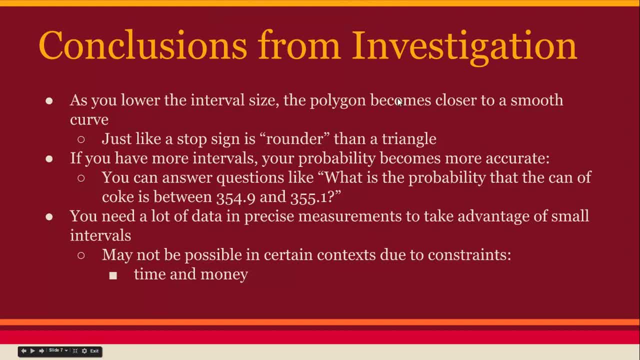 doing two days in one. but just a conclusion from that: like I want you to think about, we've got these polygons, these, these polygon graphs, but actually think about a regular polygon you can imagine, like a triangle as a wheel, and so triangle as a wheel is not very effective, but but a square is. 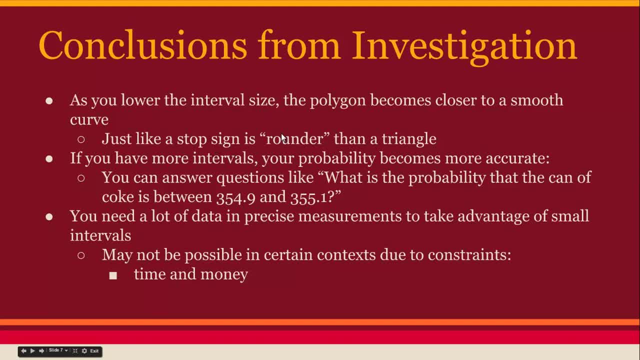 wheels a little bit better and a stop sign as a wheel. an octagon is a lot rounder. it works well. a circle is what we want. if a stop sign is eight sides, a triangle is 38 like. the more sides, the better. that's exactly we. 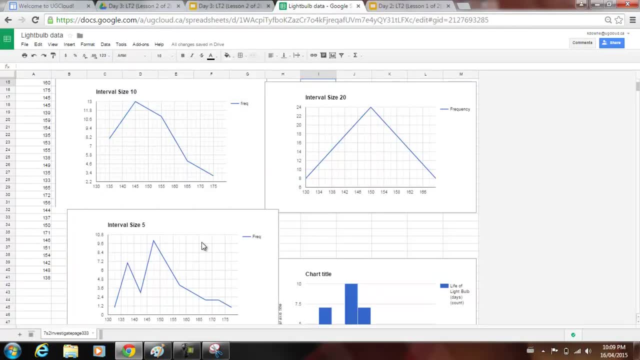 want here as well. with this data, the more sides we have, the more triangles that we're calculating, more sides we have to this polygon, the better. three is not very good. five is a little bit better. ten is even better. if we can do better than that, then we can do better. notice this light bulb data. it's just. 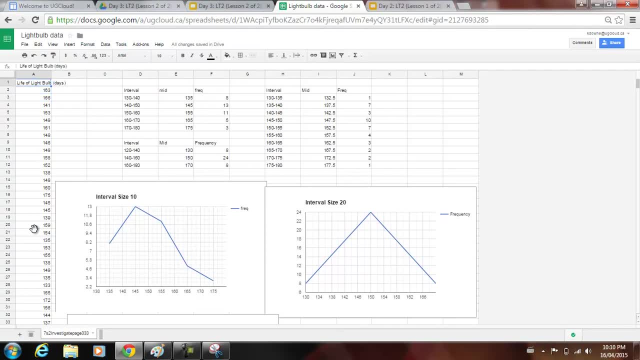 it's just the life of the light bulb in days. you can look at this data more closer in your file, but it's not calculated. there's not a lot of data here. not a lot of light bulbs were first surveyed. it looks like about 40 light. 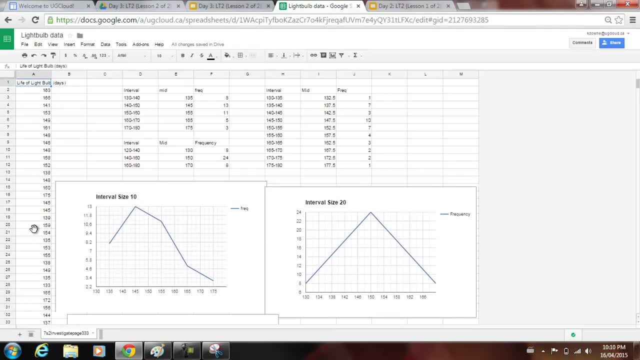 bulbs were surveyed and they didn't really calculate days more closer than just the nearest day. so if they go to do it to a decimal half a day we can get to be a lot like. we can do a lot smaller interval sizes. we have a five day. 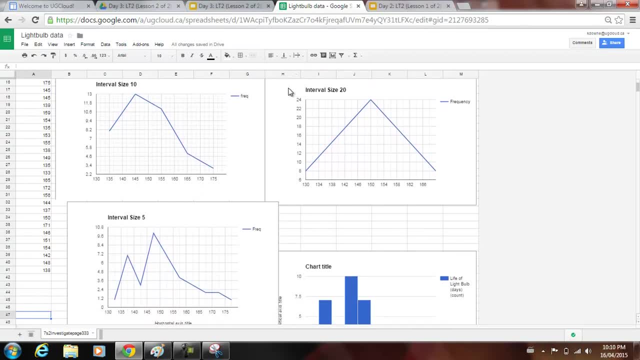 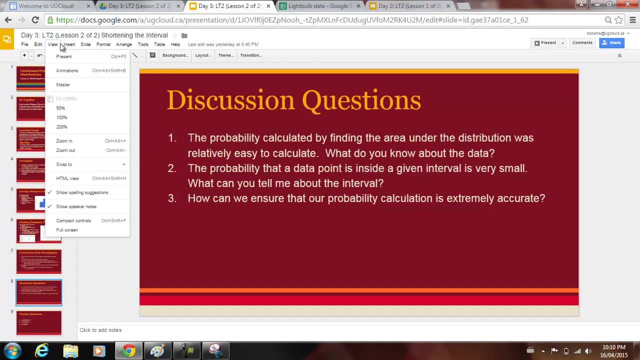 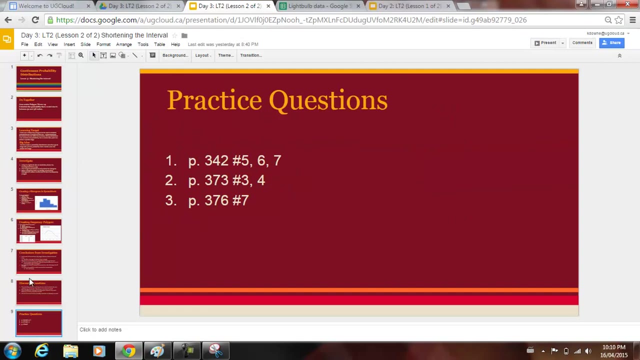 interval here. if we did a one day interval and a lot more data, then we can do a lot more intervals. ok, and that's really the point of this is really just to see, to talk about what we need to do to be able to calculate probability. sorry with that, what we need to do to be able to calculate. 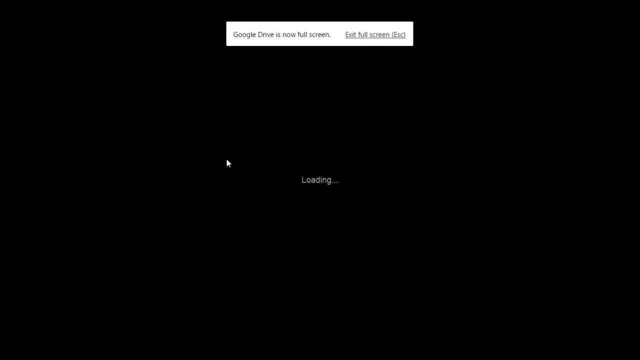 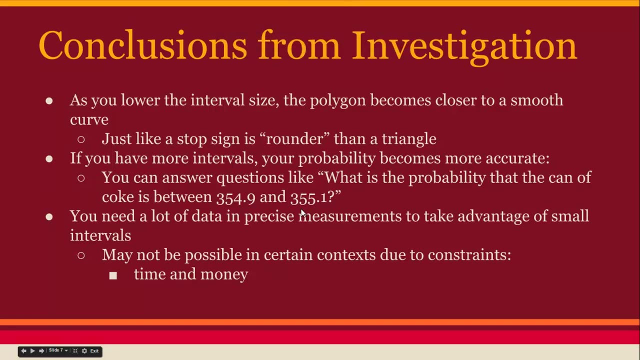 probability is. we need a lot of data. we need accurate data so we can ask questions like: what is a probability? a can of coke is between 350 4.9 and 350 5.1. if we have have a lot of cans of coke and they've been very accurately measured, we can answer questions.